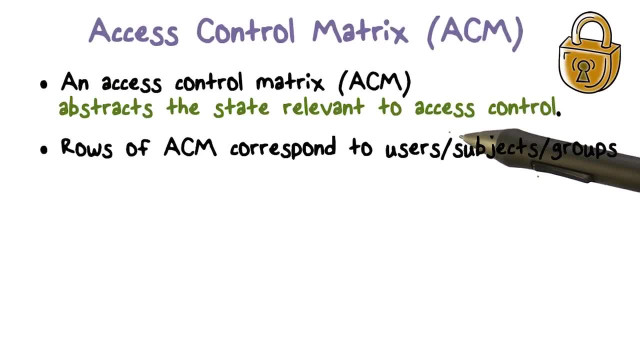 To define a matrix you have to say what rows it has, what kind of columns it has, what does it store in each element or each cell of the matrix. So an access control matrix. rows are defined by the users or subjects that we have in the group. 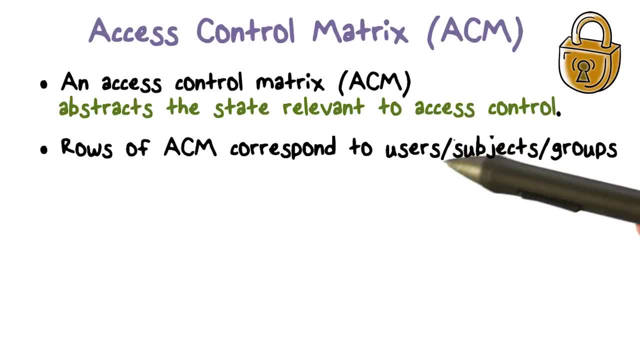 So rows actually correspond to the sources of requests, or the subjects or the users. So this access control matrix, Alice is a user in the system. There is going to be a row for Alice. Well, other thing that a matrix has to define this two dimensional matrix, we 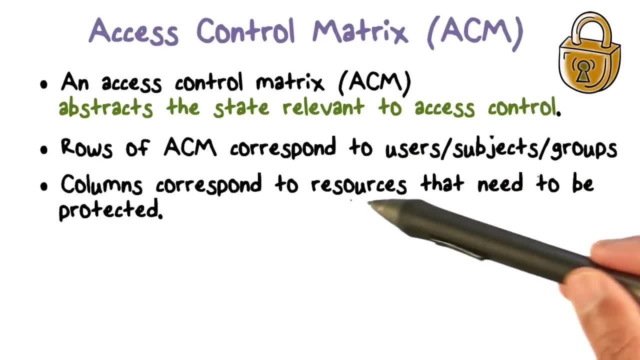 are talking about is we have to define its columns. Rows correspond to users, Actually columns going to correspond to resources that we have in the system. So each resource that needs to be protected, Remember, we need to know who's allowed to access it or not. 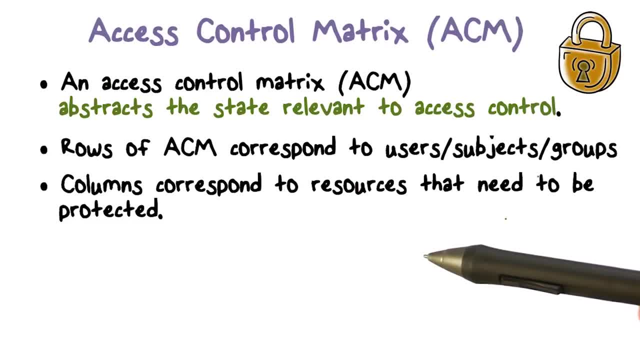 So this matrix is sort of telling you for a given user, that's a row and a given resource or object. Okay, What can be done? So the columns are going to correspond to all the resources that need to be protected in the system. 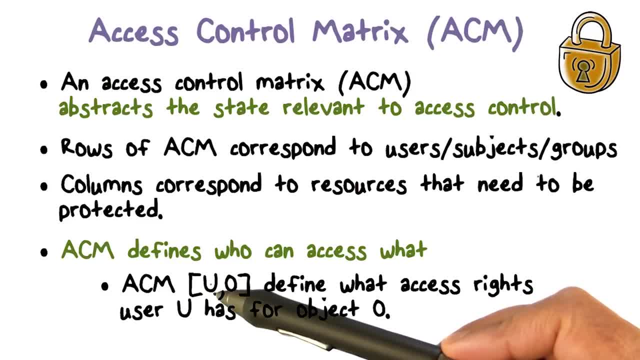 So an access control matrix. since I'm talking about rows and columns and it's two dimensions, any particular entry or cell in this matrix can be defined by what we have here: u, o, where the row that is corresponds to user u. 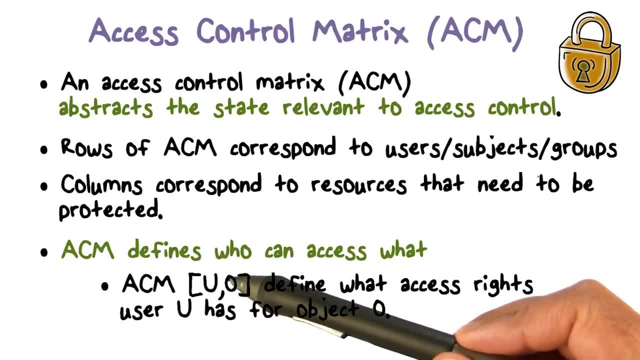 and the column for object o. So you start with a user, continue until you get to the object that we're talking About. so that element of the metrics, or cell with the metrics, is actually going to define what kind of access rights user u has for object o. 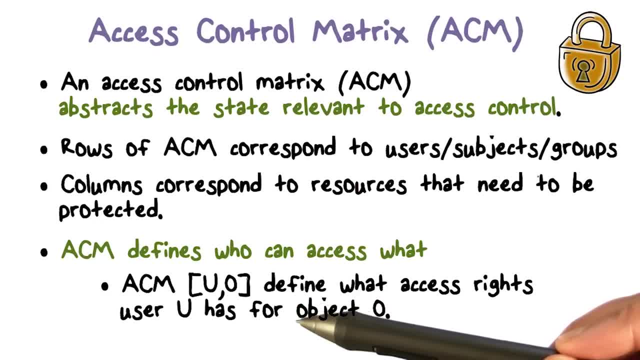 So if this was a file and access rights can be read, write, execute whatever subset of those access rights, Then we saying the entry in the matrix. if you look at the row for user u and object o, it's going to say if you can read this object o. 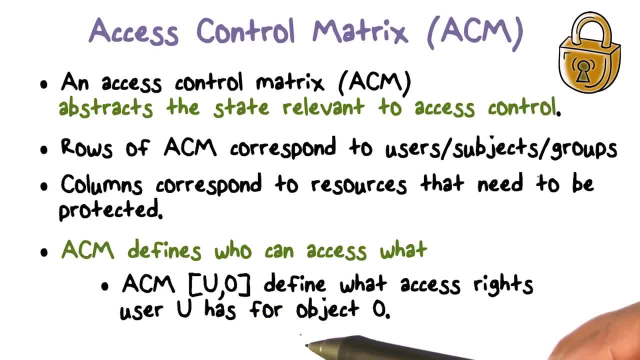 R is present in that entry. That means the user can read object Matrix. access control matrix is based on users we have in the system, resources we have in the system and the state actually it captures is who has what kind of access for the resources of the system. That's what each entry of